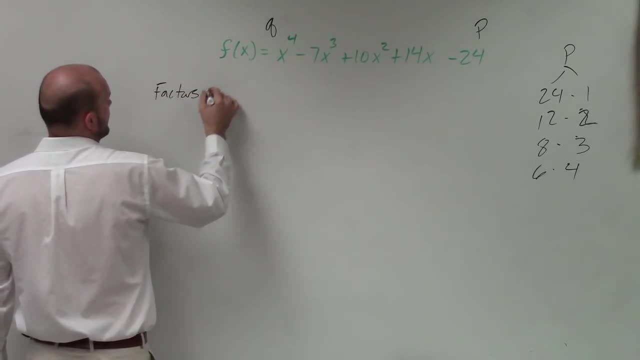 p over q. remember, it's the factors plus or minus p over q. Well, my q, the coefficient of q, is 1.. So we know, the only factors, Justin, of 1 are 1 and 1, right, So therefore, it's going to be 24,. 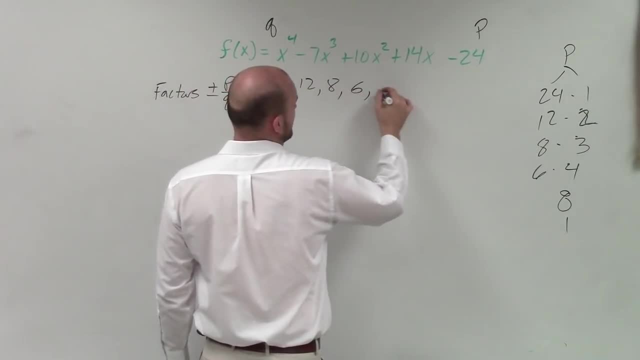 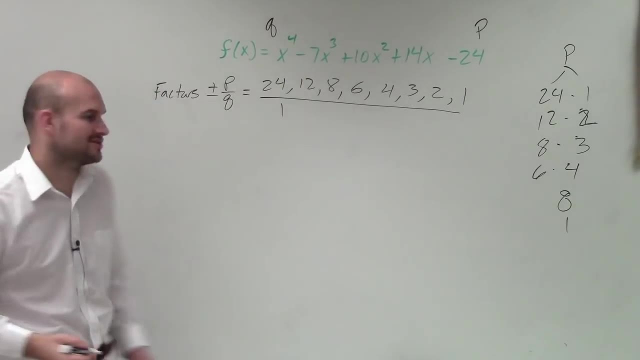 12,, 8,, 6,, 4,, 3,, 2,, 1, all over 1.. So when doing my factors you can say: well, all the possible rational zeros, p over q is just going to be plus or minus. Now you can write plus or minus. 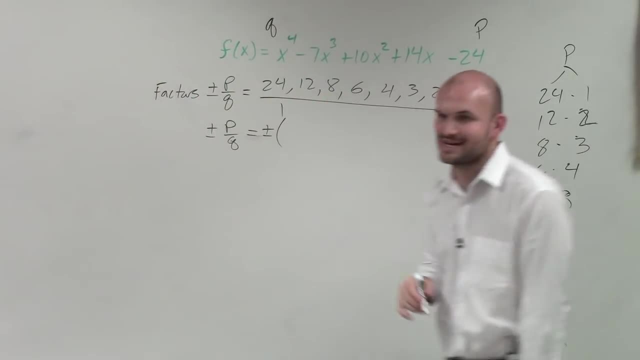 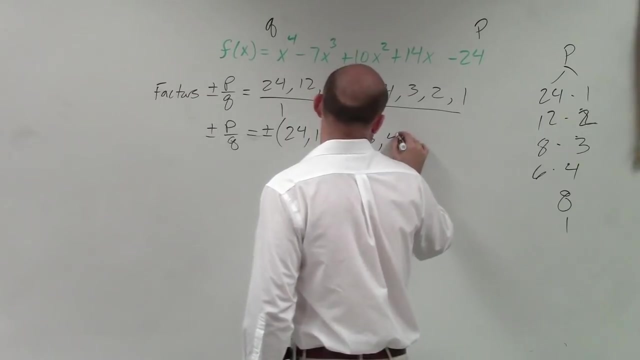 for every single term, if you want to. Or you can also just put plus or minus outside of parentheses and say plus or minus. So you can just put plus or minus outside of parentheses and say plus or minus is going to be distributed to all of them And just write them as 24,, 12,, 8,, 6,, 4,, 3,, 2, 1.. 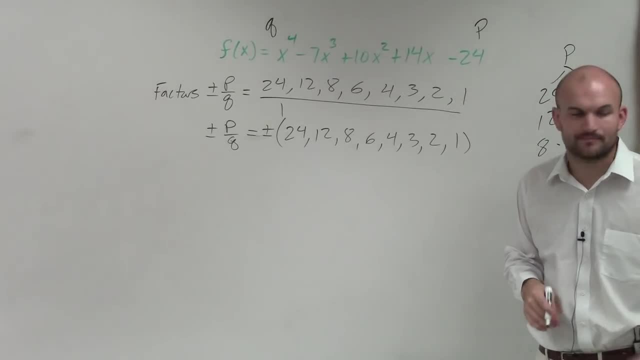 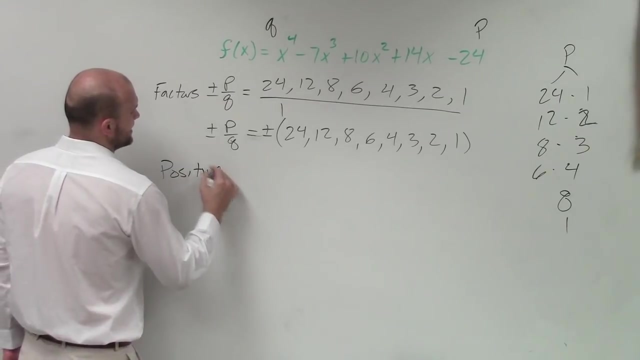 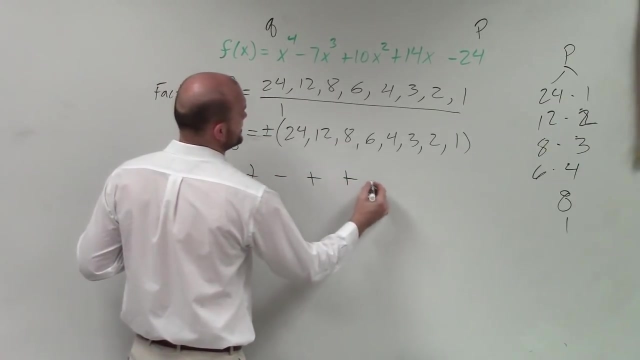 OK, Very good, OK. So now let's go ahead and determine the positive real and negative zeros. So when I take a look at the positive, I'll just take out, I'll just written down the positive, take out the signs goes to positive to negative, to positive to positive to negative. right, All I? 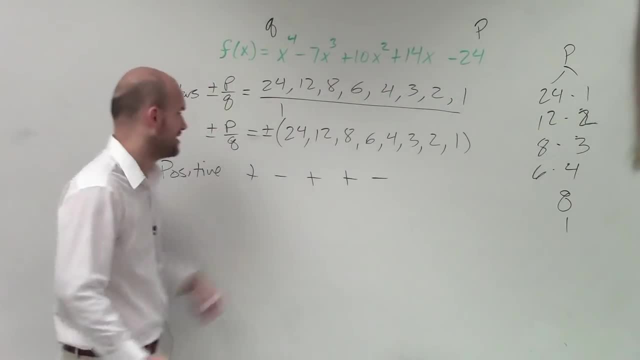 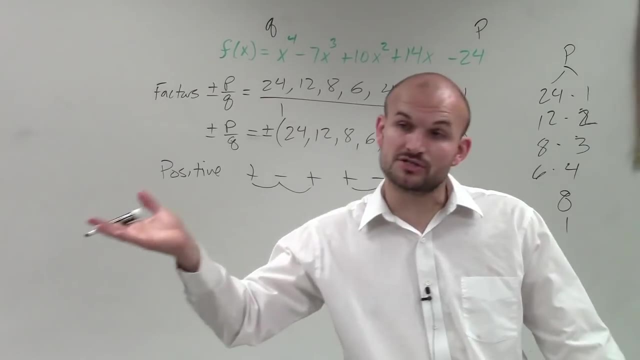 did was I took the sign of each one of my monomials and I brought it down. Therefore, you can see I have three of them, right. So 3 minus an even number, 1 even number is 2.. So 3 minus 2 would. 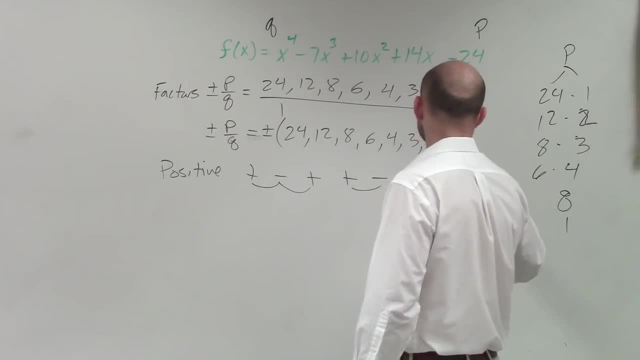 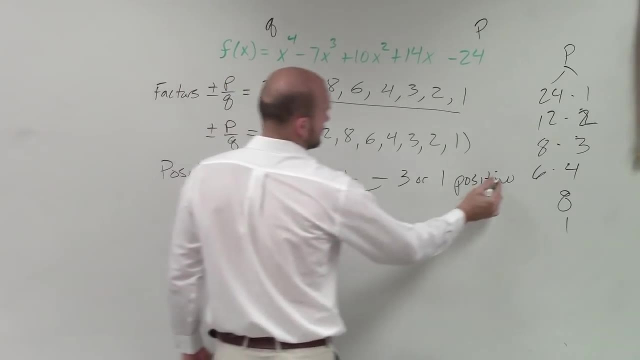 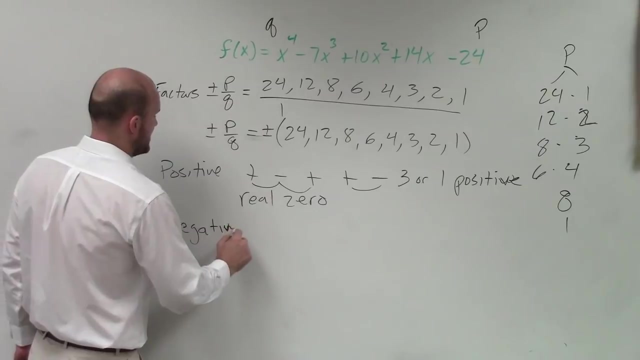 be 1.. So therefore, I have 3 or 1 positive real 0, correct? OK, Now let's go and look at the negative. Now I'm going to kind of do this in my head because I already showed you guys what to do. Yes. 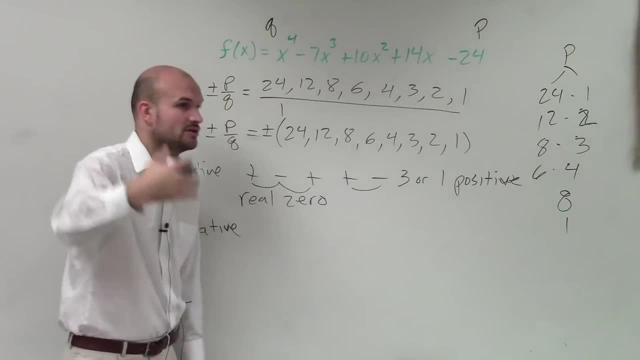 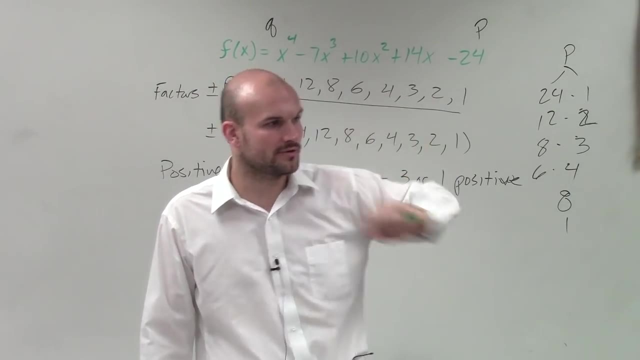 Do you always subtract 2?? Yes, You can keep on subtracting. So let's say I gave you 10.. Let's say there's 10 alternating signs. Then the number of possible real zeros would be 10,, 8,, 6,, 4,, 2, and 0.. OK, 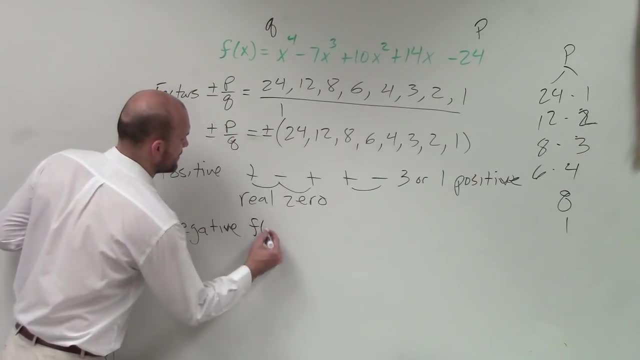 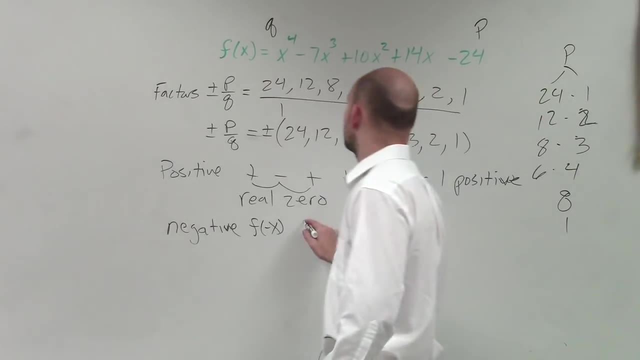 So now let's go and look at the negative. Now remember the negative. you need to evaluate for f of negative x. To keep this video a little short, I'll do the signs out here. So that's going to be positive, That will be positive, That will be positive, That will be negative And that will. 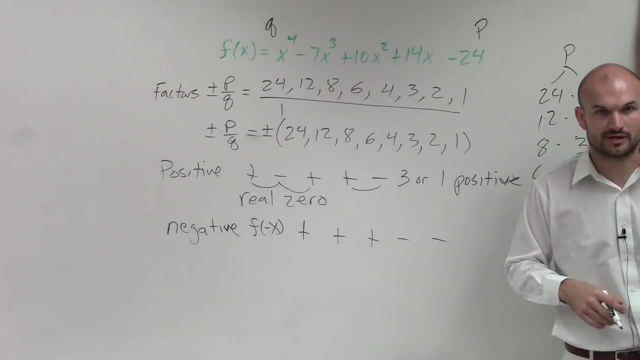 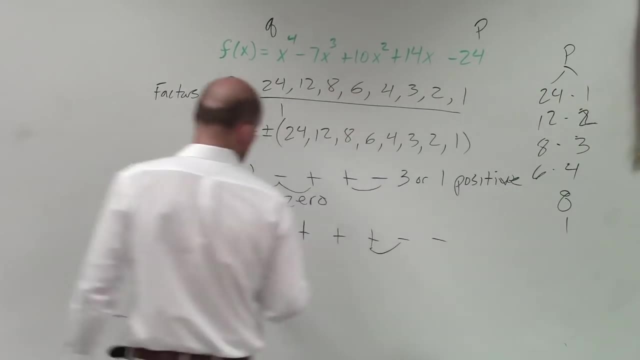 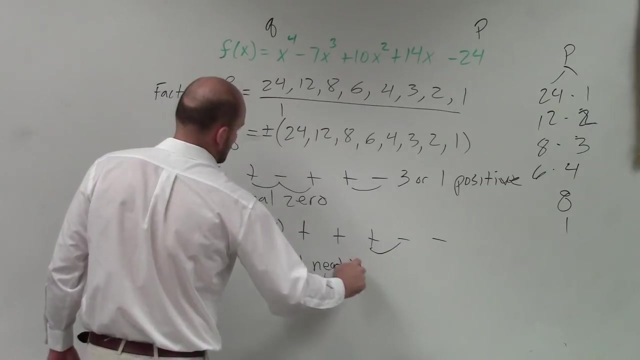 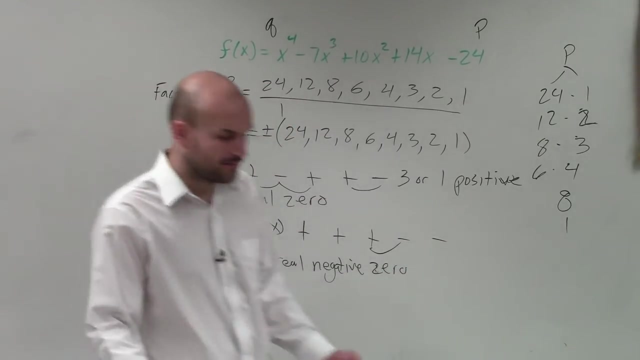 be negative. I did this in my head, OK, You guys can check my work, But you can see that there's going to be one alternating sign, All right. So therefore, we'll have 1 real negative 0. OK, So what we have right now, ladies and gentlemen, I'm asking you to find the zeros, OK. 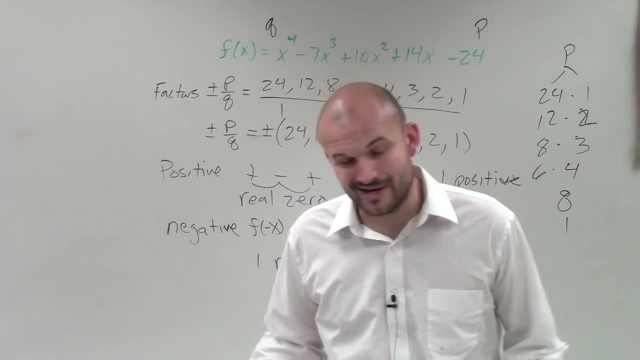 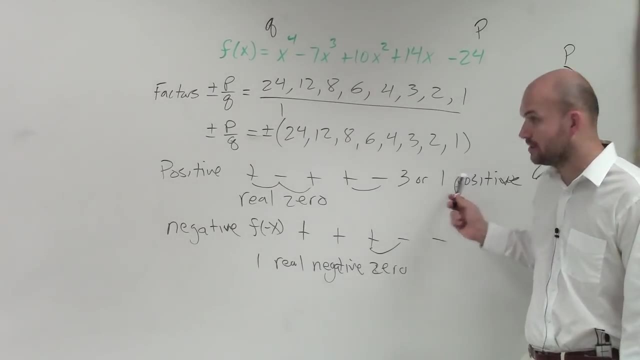 I'm asking you to find the zeros. Let's say you don't have a graphing calculator, All right, And you're not allowed to use your phone for Google. So I say you're going to have three positives and one zero, or one of them is going to be negative. And if it's rational, here are all. 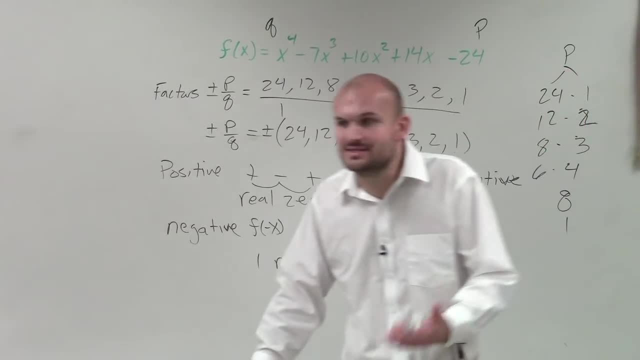 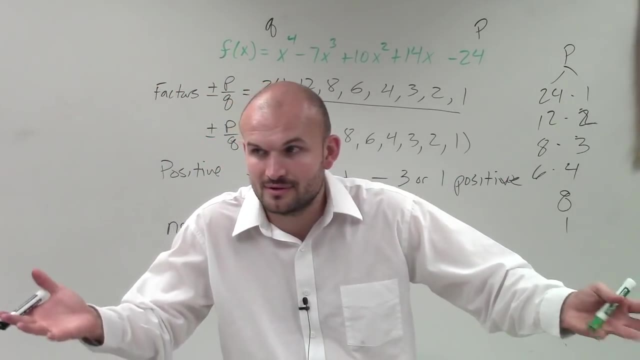 your zeros. So how do we determine if something is zero? If we're given a zero, how can we determine if it's a zero of a polynomial? It kind of goes back up to what we said earlier. So we're going to look at my first problem I did today. What can we do? We can do how we can determine if I give. 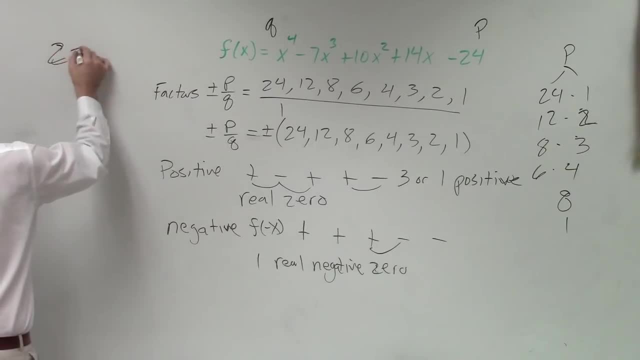 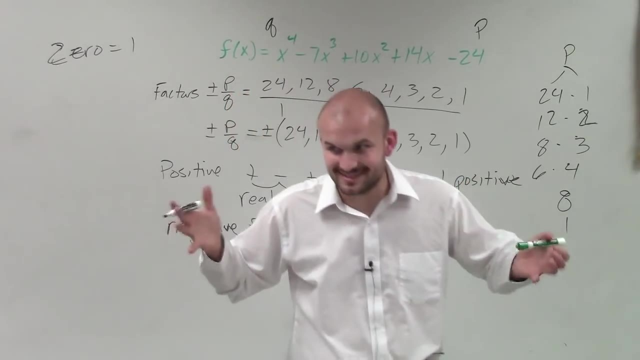 you a zero. if I say a zero, if I say zero equals 1, how do you know that 1 is a zero? What can you do? What process can we do? Yes, You can plug it into the equation, right, And if you plug it into, 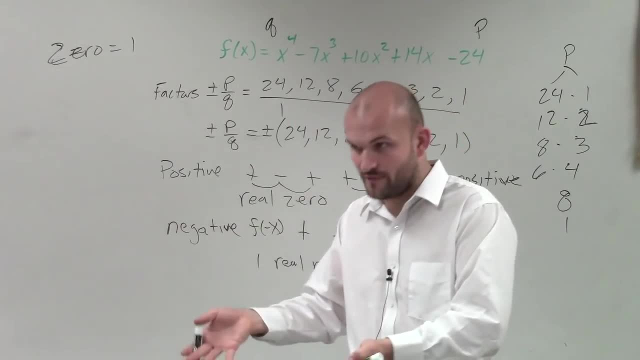 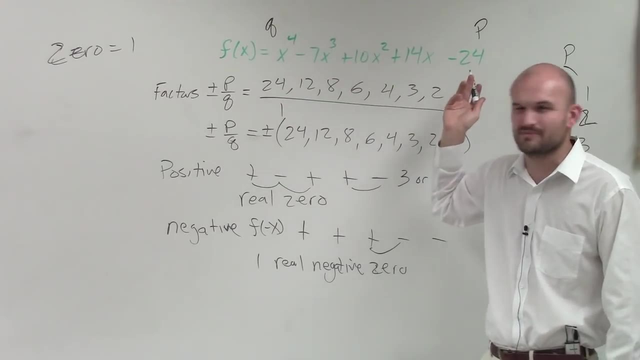 the equation and you get zero, then you know it is a zero of the function. right, Very good. However, if I get up to like 24, I'm probably not going to want to plug 24 into this. It's just going to be a. 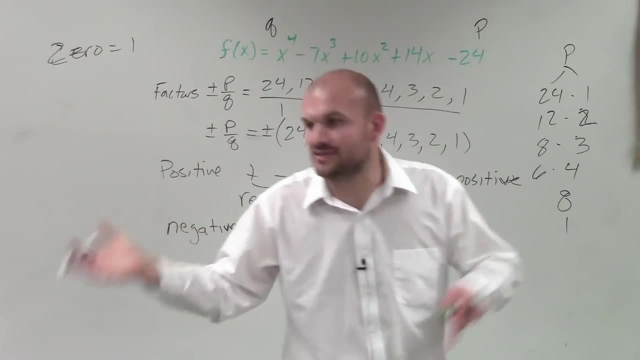 math, right. And then plus, what do I do after that? How is that else going to help me? So let's say you plug it in and you get a zero. Well, all right, so that tells you it's a zero, but what do? 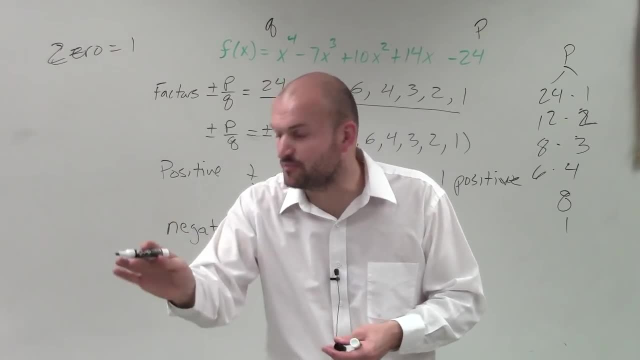 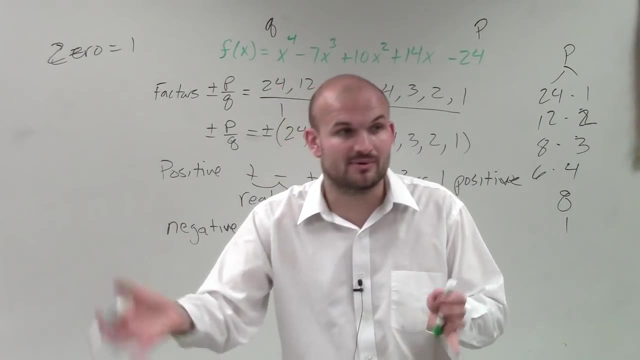 you do from there. So what else can you determine the zero? Because plugging it in is a great way to determine it. but there was another way that we determined: by using the remainder theorem. right, The remainder theorem was plugging it in, but then we could also check it by what process I did it. 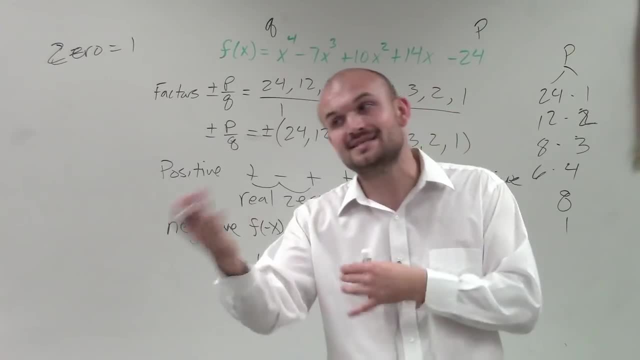 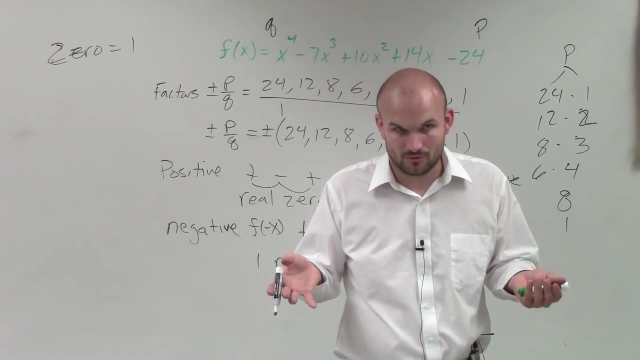 today, synthetic division. And what's nice about synthetic division? it's the exact same thing as what you said. but when you do synthetic division, what do you get? your answer You get. your answer is what we call the what Quotient. And that quotient is what of the polynomial A factor. 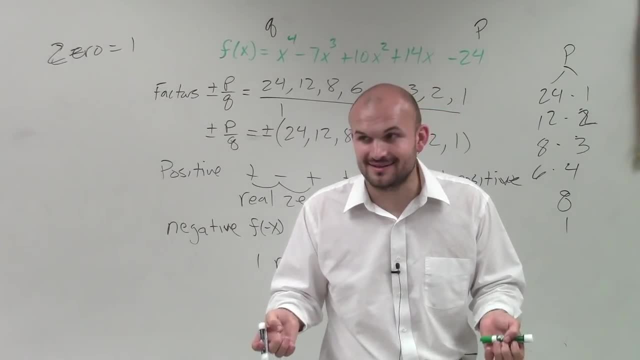 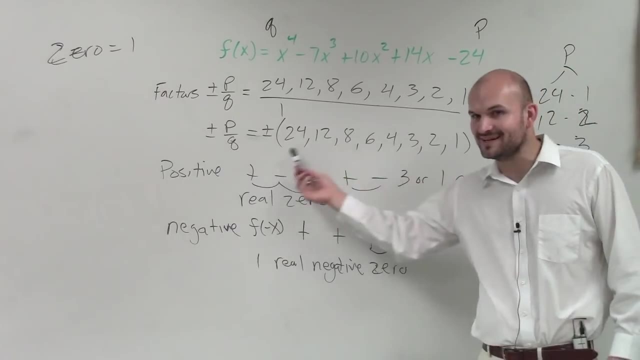 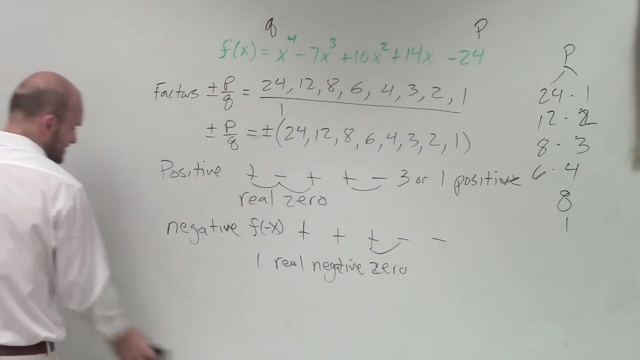 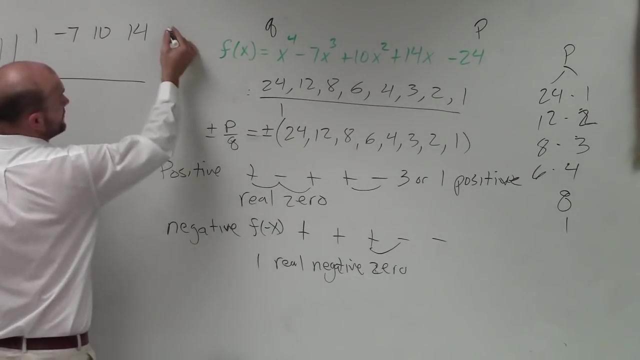 And from a factor we can find what The remaining zeros, right? So here's the problem, though I don't know which one is a zero or not, right? So guess what? If you don't know what the zeros are, you're just going to have to check. So if you don't know what the zeros are, guess what. 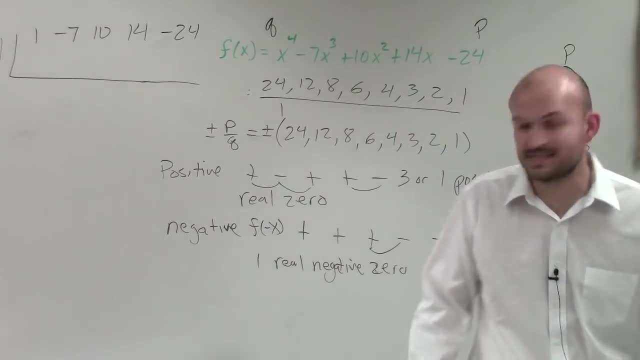 ladies and gentlemen, You're just going to have to guess and check. Why start with the heart? Why start with 24?? Let's do the easy one: 1.. Once you say 1, it's probably pretty simple to start, And 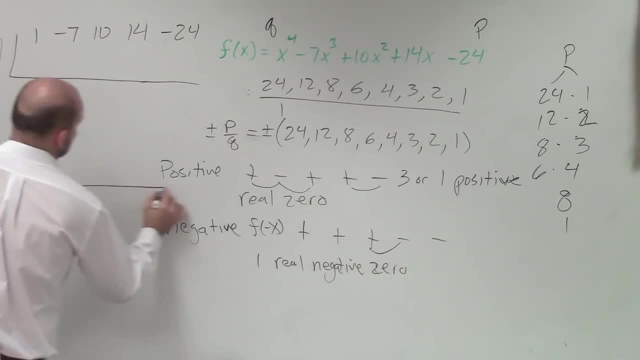 then if 1 doesn't work, we'll do negative 1, right, So let's do 1.. Bring down the 1.. 1 times 1 is 1.. Negative 6, negative 6, 4, 4, 18.. So that doesn't work. 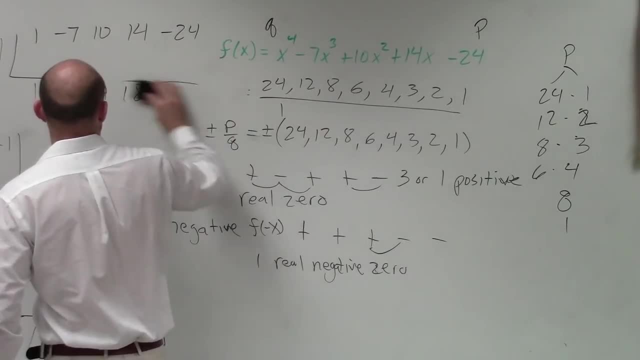 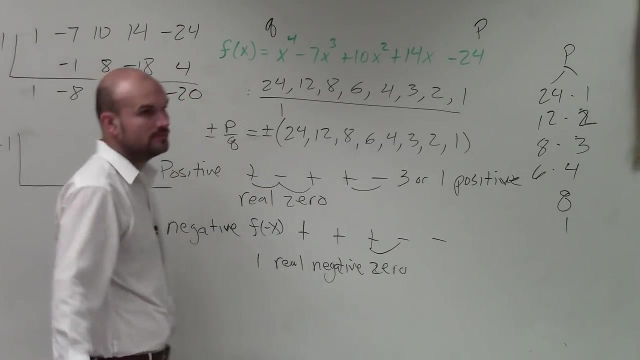 right. So you go back to the drawing board and say, OK, that didn't work, Let's do negative 1.. So you bring it down. So negative 1 doesn't work. So what do you do? Negative 1 doesn't work. 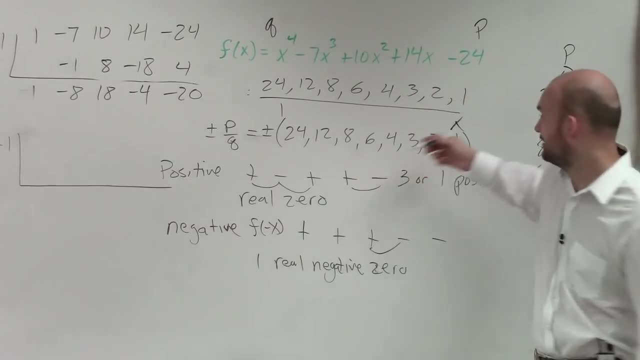 I'd move to 2, right, And then do it both for 2 and negative 2.. Then I'd move to 3 and try 3 and negative 3.. Now I use graphing technology and I know that 3 works. So if you didn't use graphing, 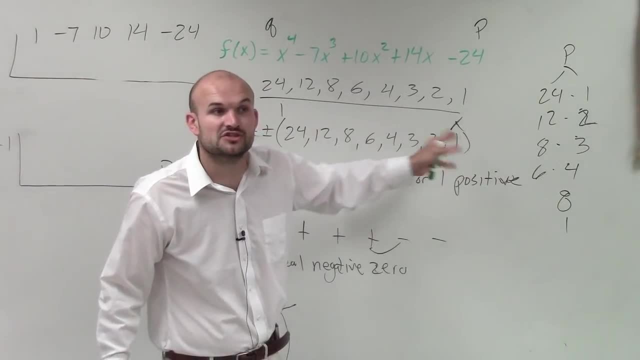 technology, you'd probably be a couple minutes behind me because you'd be doing synthetic division for all of these until you got up to 3.. So I do 3.. Bring down the 1.. 1 times 3 is 3.. 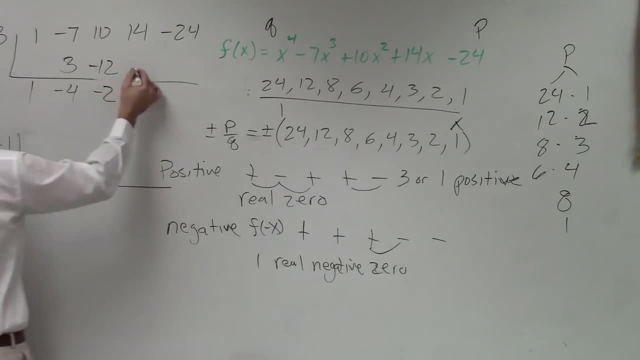 Negative 4, negative 12, negative 2, negative 6, negative 8.. No, no, no, it's positive 8.. Positive 8.. Yes, OK, So now that's nice. So now I have a. 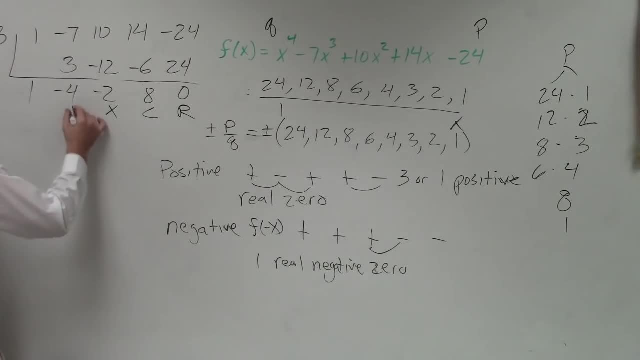 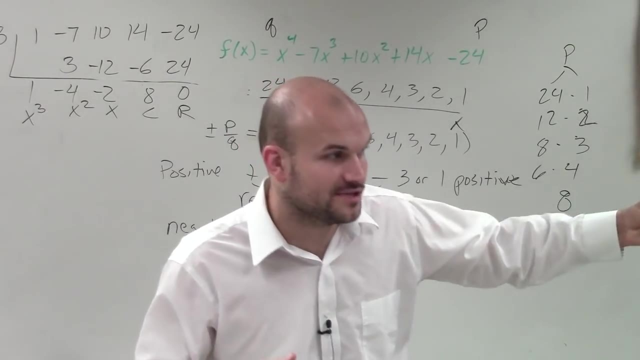 polynomial. Remember remainder constant, linear, quadratic and cubic. But now do you guys remember when I gave you that 1, 0 and I applied synthetic division And I said: hey, once you have 0,, then you can keep on doing it right? OK, So we know that 1 is not a 0.. We know that. 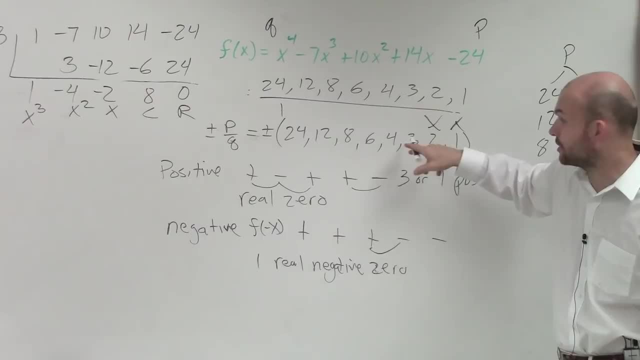 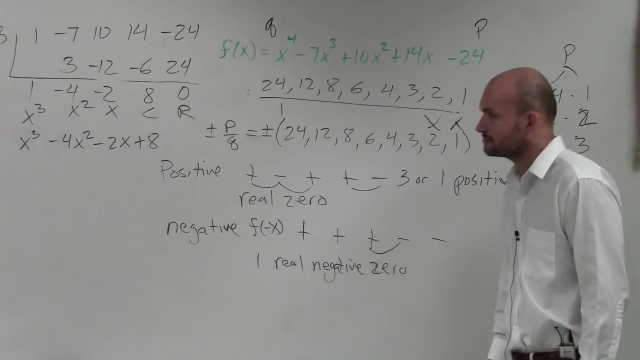 2 or negative. 2 is not a 0. Now we know 3 is a 0, but you can either try to factor this, So you can say: is this quadratic or not quadratic, but is this factorable? Is that factorable? And you could. 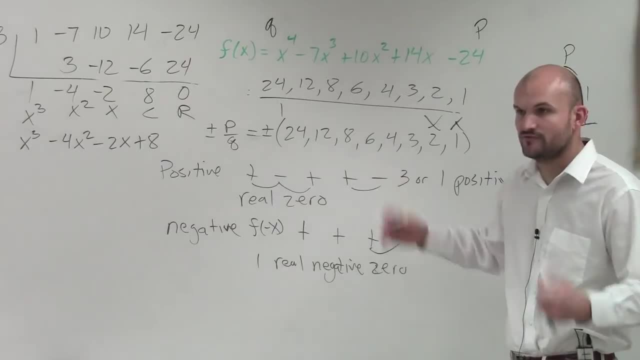 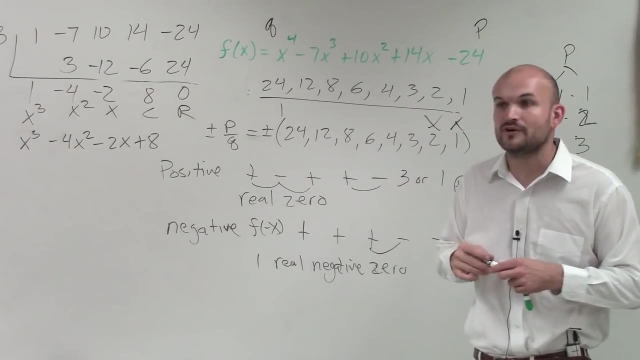 factor it by what? Grouping? right, OK, Now you could factor that and be able to determine. So here I would be able to factor out. Yeah, you can go and factor that by grouping, It wouldn't be a problem. However, if you use your graphing technology, you're going to be able to factor. 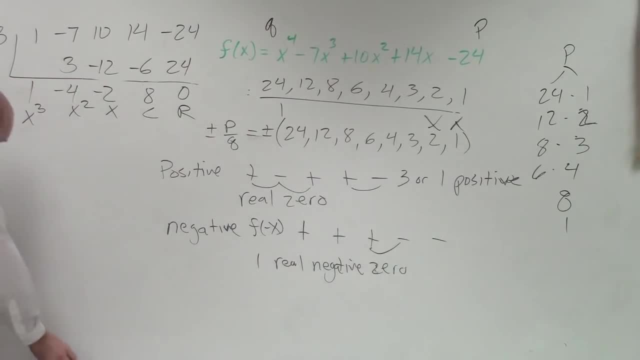 that out. So if you use your graphing technology, you would also notice that 4 is also a 0.. So, rather than factoring it, I already know that I use graphing technology, so I know that 4 is also a 0. And I'll show you guys how to determine that with your graphing technology. So, rather than 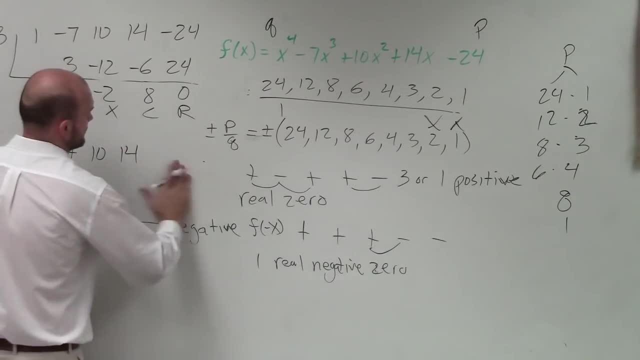 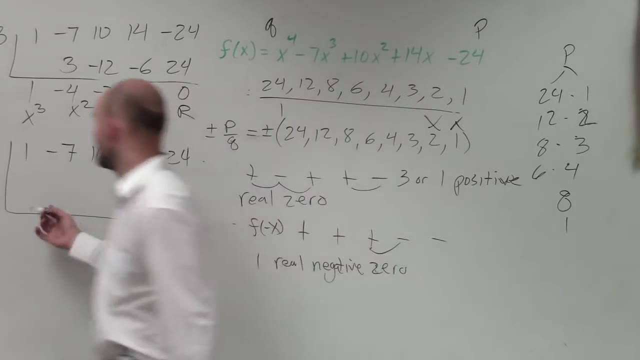 factoring, because maybe I'm just not good at factoring so I don't want to do it. So I'll go and factor it again By doing synthetic division. I bring down the 1.. 1 times 4 is 4, negative 3,. 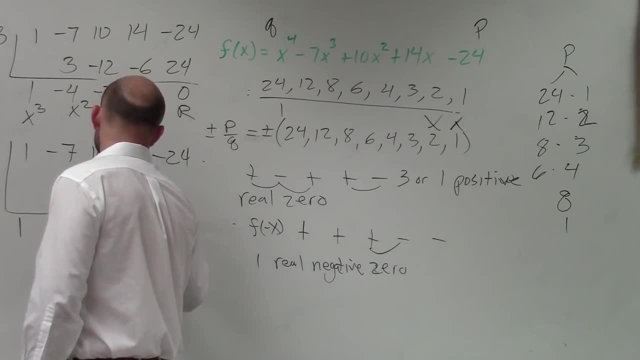 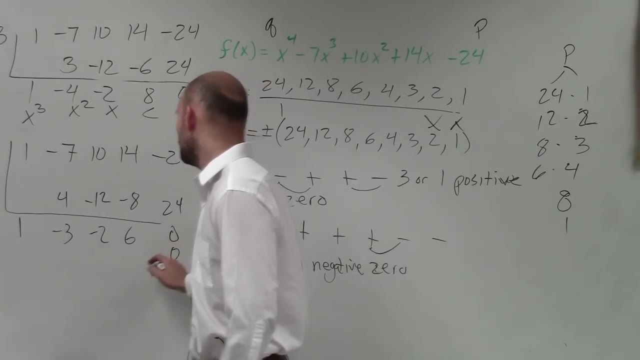 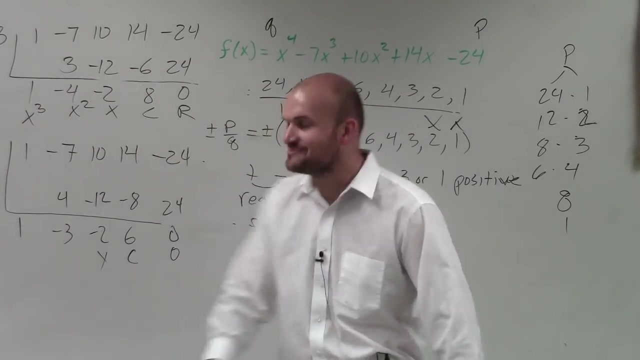 negative 12, negative 2, negative 8, positive 6, 24, 0.. Now I have a 0 constant linear. Did I pick the wrong one? I rewrote it All right, big mistake. You don't want to make sure you do this. 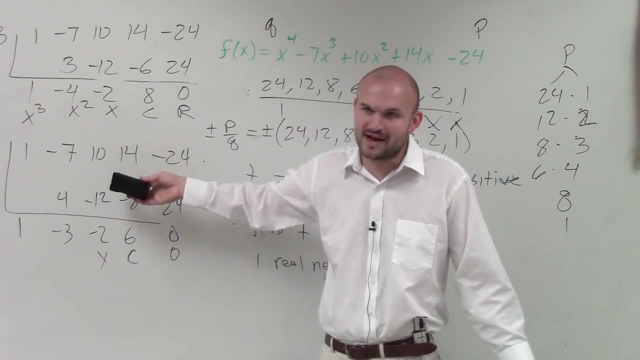 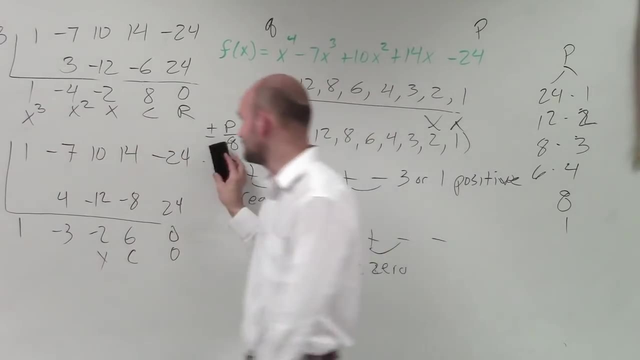 If you guys notice, if I rewrite the factor, same thing, I'm just going to get another factor. I'm not simplifying at all. When you refactor you have to take your previous quotient and then do that down further. My mistake, Sorry about that, Because you guys notice when I did that. 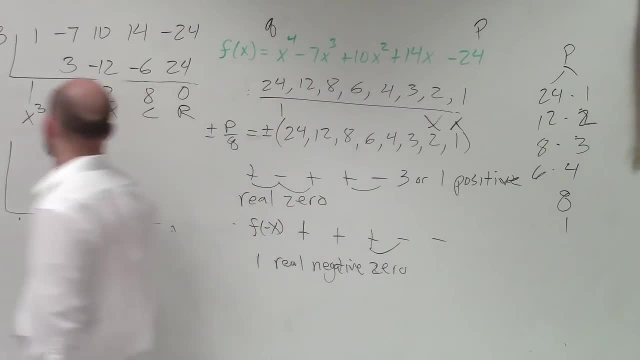 again I'm getting a factor to the third power. So take 1, negative 4, negative 2, and 8.. Bring down the 1.. 1 times 4 is 4, 0.. 0 times 4 is 0, negative 2, negative 8.. All right, Therefore. 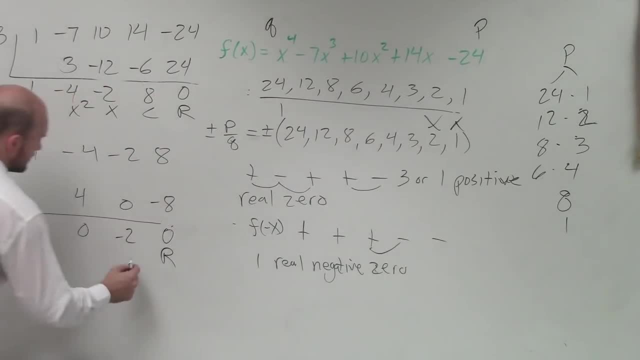 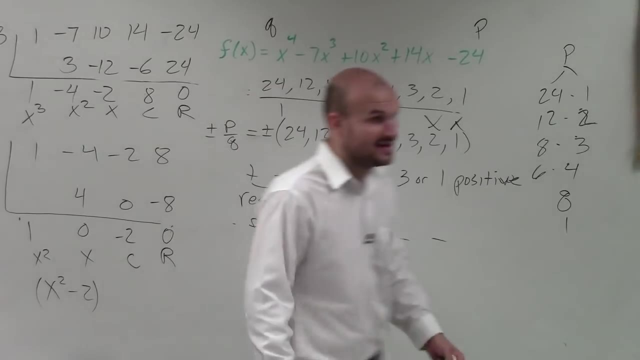 that becomes 0.. Now, you guys see, you have a remainder constant linear quadratic. So you have x squared x squared minus 2.. That is your factor, right, And can you solve the other two 0s by using that? 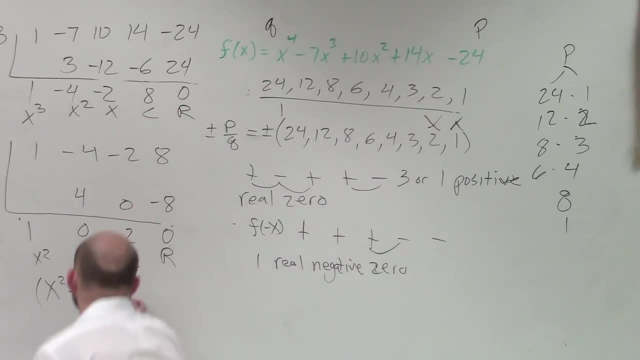 factor: Yes, So let's go and do it. We set it equal to 0.. I'll do it over here: x squared minus 2 equals 0.. x squared equals 2.. Square root: square root x equals plus or minus the square root of 2.. 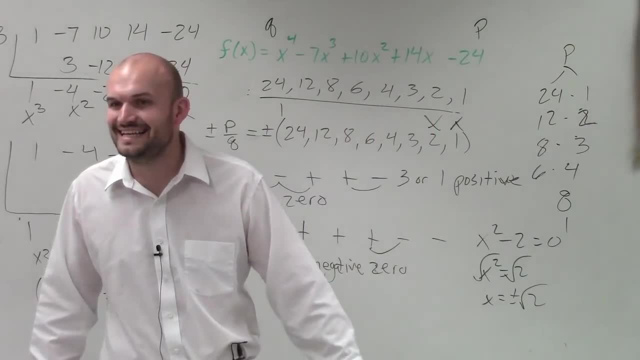 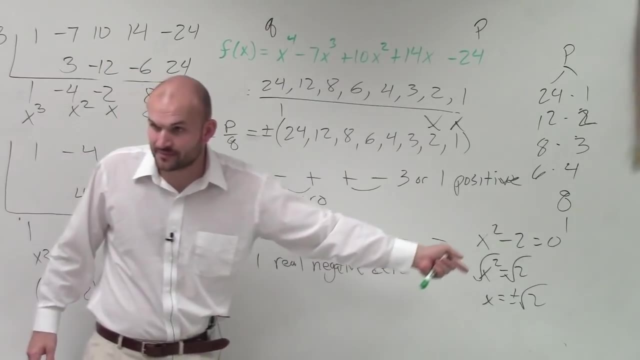 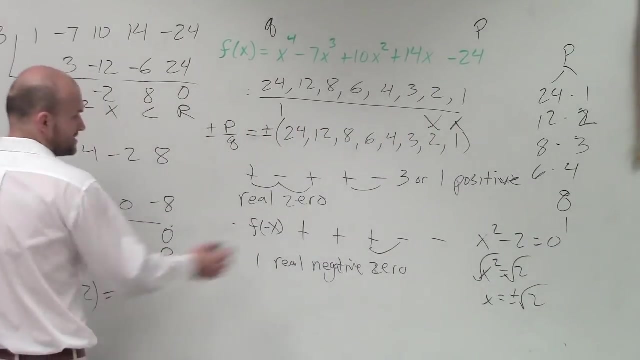 Now is the square root of 2,. is that a rational number Or is that a irrational number, right? So that's why square root of 2 is not here, because it's not rational, It's irrational. Now let's count the number of 0s. We have the 1, 0, which is 3, right? So we know those are 0s. 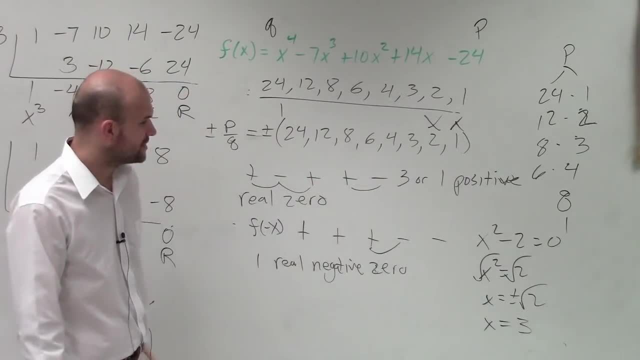 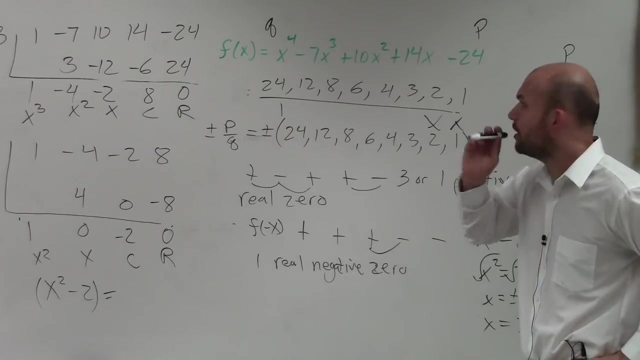 and also: x equals 3.. How many positive 0s do I have? 2. That's issue. So I'm missing a 0. 3. No, Oh, I'm sorry, And I forgot to write down that one. We said 4 is a 0 as well, right. 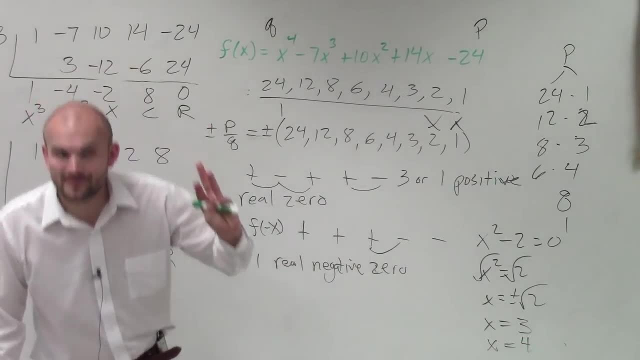 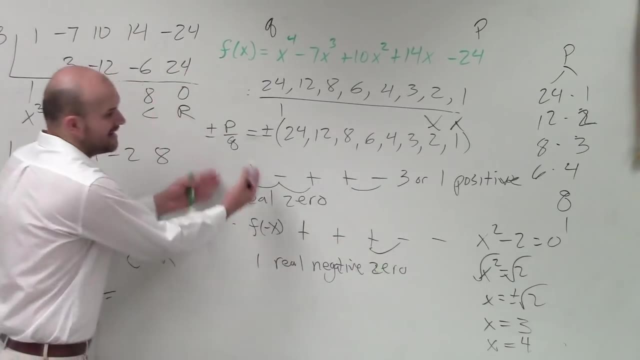 So how many positive 0s do I have 3.. How many negative 0s do I have? 1.. And are those real? Just because it's irrational, it's still real, right? So you guys can see it follows this case. 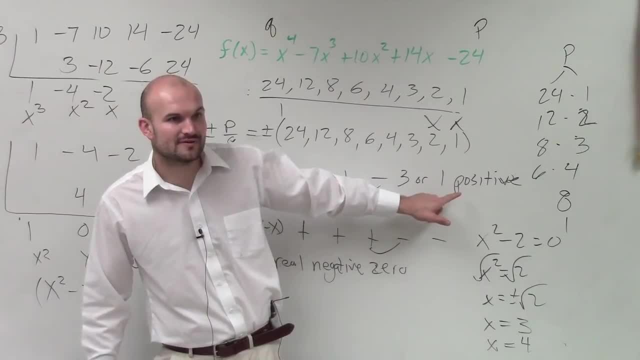 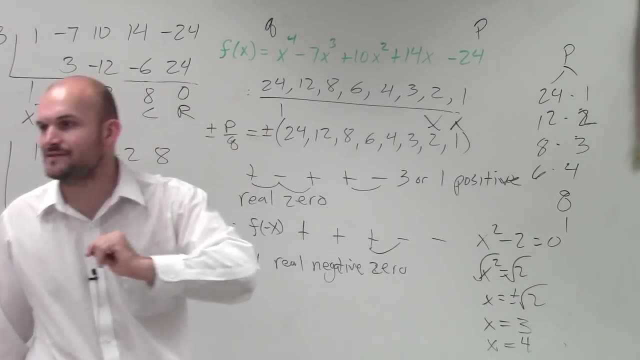 Now, however, let's pretend I only had one positive. If I only had one positive and I only had one negative, that means I still am missing two more 0s. If they're not real, then they have to be imaginary, okay. So in this problem, though, we have all real 0s, which is cool. 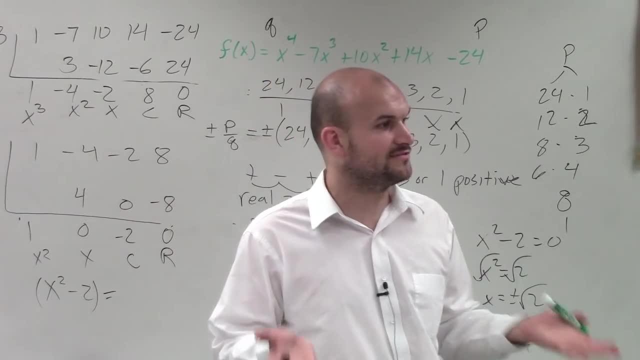 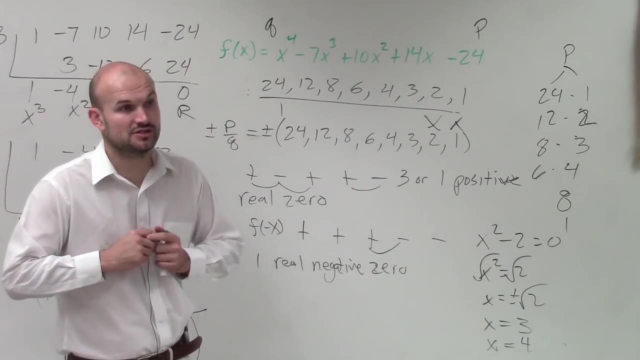 though that by using Descartes' real signs. if you don't have enough to count up the real, that means the other ones are imaginary. Yes, Do we have to find the 0s? Yes, You will have a problem, just like this, using graphing. 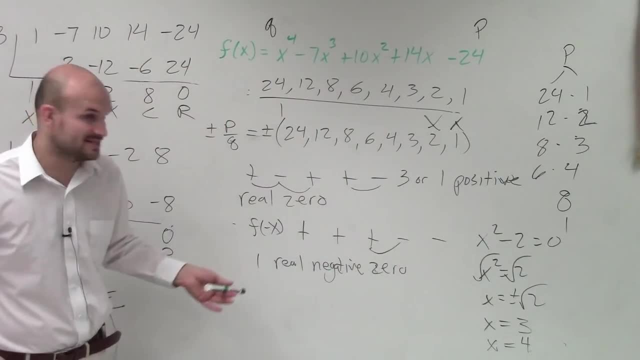 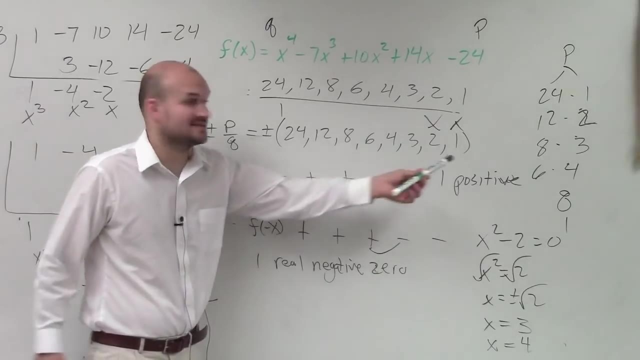 that you'll either have to do synthetic division until you find the 0s or use graphing technology. Yes, You'll have to start from the lowest and then every time you go up, Yeah, I mean you can start from the highest, but yes, I would recommend starting from the lowest. 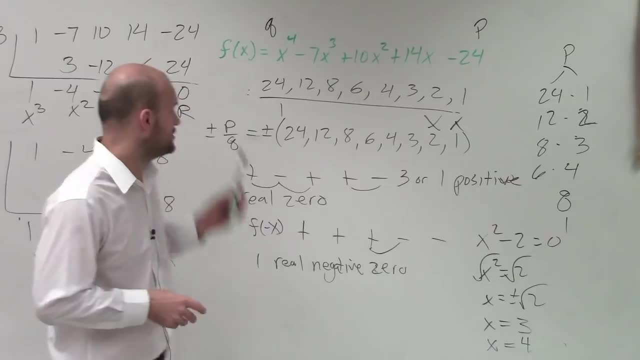 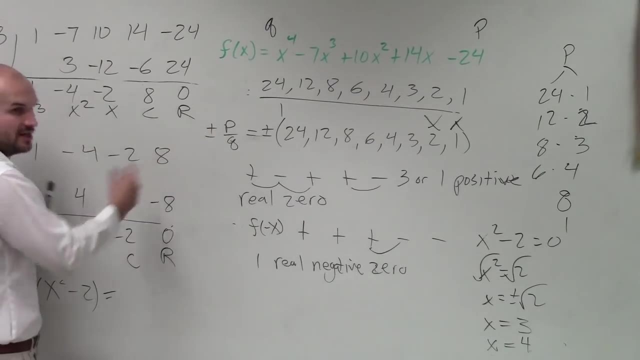 And then every time you go up that thing you put it in a different one, Yeah, then you find, Once you figure out one, 0, then you take, Yeah, Yeah, You take the quotient and then you keep on working the synthetic division until you find another 0, okay. 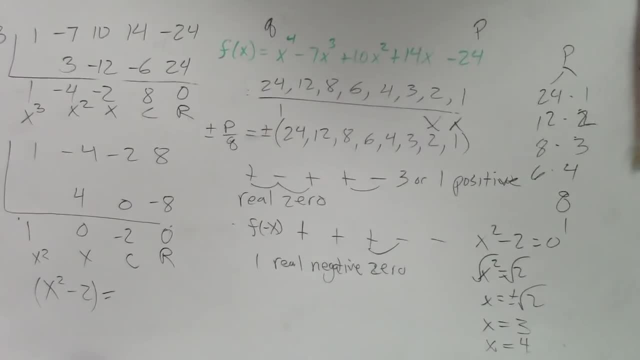 Now I'm going to talk to you, though, about your graphing calculator, how you don't have to do all that legwork.